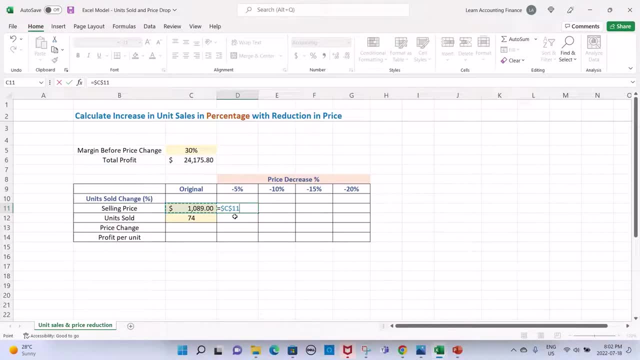 so i press f4 and i freeze the cell reference so that it doesn't move as i move the phone and i basically apply the formula. okay, so the new price is 1 plus whatever your price change is. okay, so in this case it's negative five percent. i'm linking so that the model works, even if we 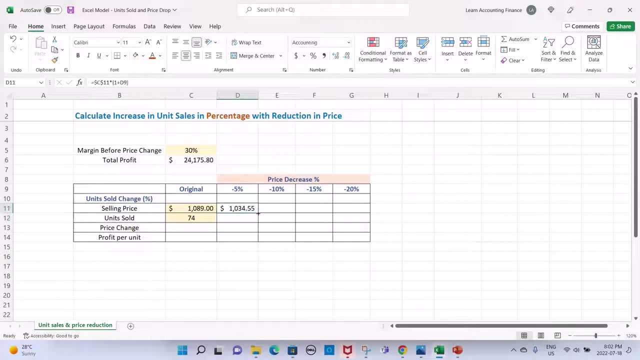 change the inputs. okay, so i press enter and you see that the new price is 1034. drag it all the way to the end and you have prices for each change in percentage. okay, now that we have the selling prices, we can also calculate the change in price and the profit per unit, right? so let's go ahead and 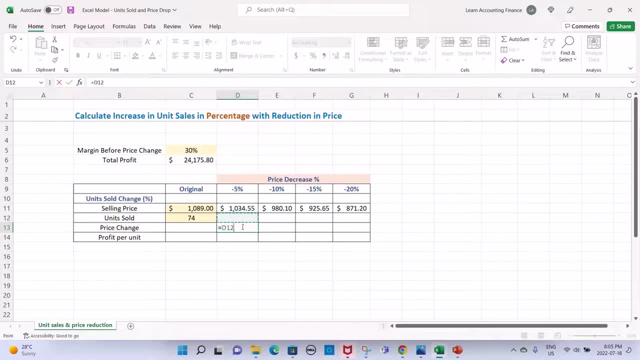 start with the change in price. so this will just be a difference of our new price and our original price and again i will freeze the cell reference for the original price so that we can carry this over to the other columns originally without any change. our profit per unit is calculated as: 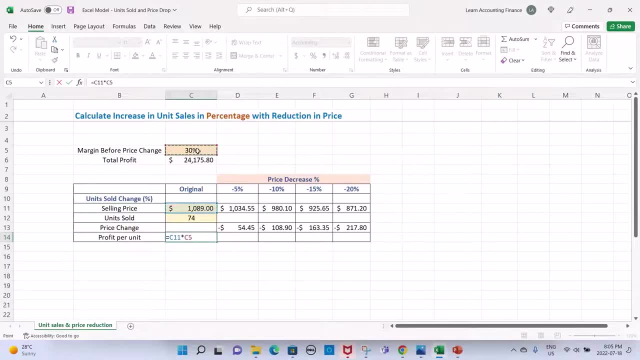 selling price times margin percentage. this is the profit per unit. in a way, you can also indirectly calculate the cost. so really, if you wanted to calculate the cost, that would be the difference of your selling price and your profit per unit and this is really your cost now for the profit. 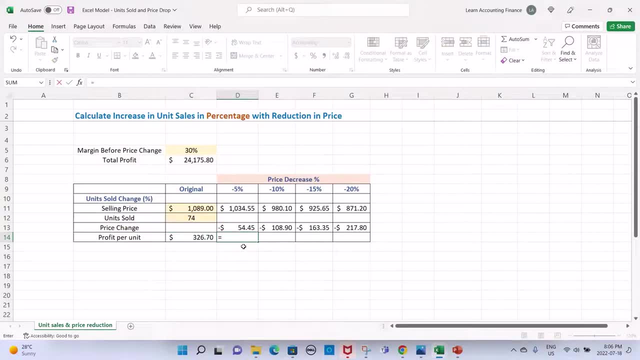 per unit for the revised prices. that will be the difference in price. so your original profit per unit plus the change in price will give you the profit per unit for each of these different price levels. and this is because we are not changing the cost. the only thing that is changing is the. 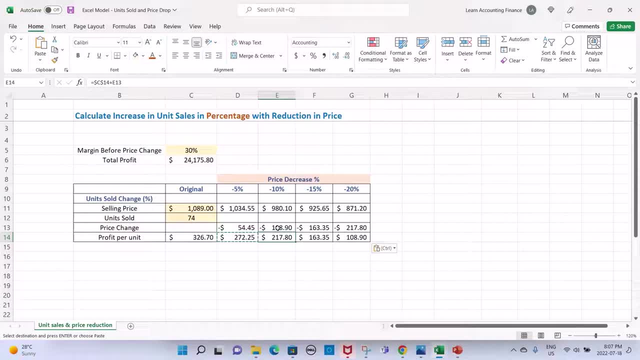 selling price and this will have a direct impact on our profit. this will be a direct reduction of our profit at each price change level. now we will calculate the quantity of units sold on revised prices. so this will be our total profit, the original total profit because, remember, we do not want our total profit to change at these price levels. that's why the 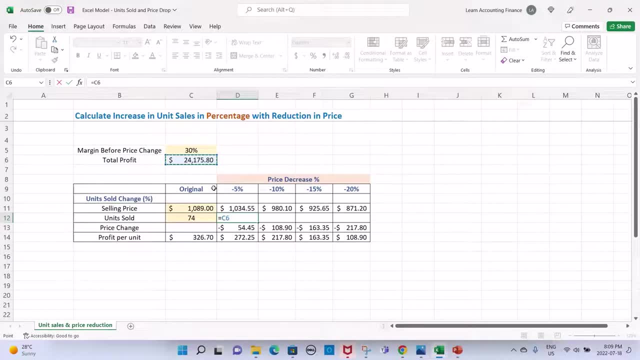 units will change. when we reduce the price, the number of units to be sold needs to increase so that we can still achieve this profit despite the drop in profit per unit. so original total profit divided by the new profit per unit. this is important. this will calculate the number of units required to